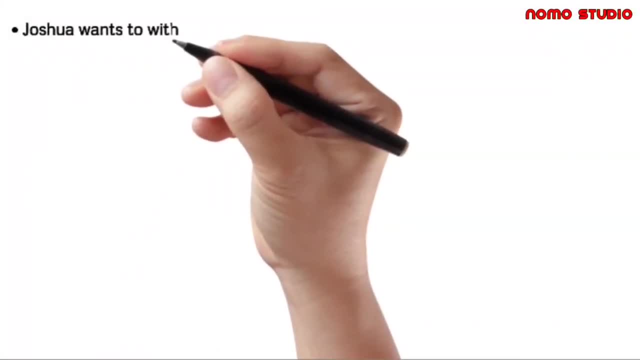 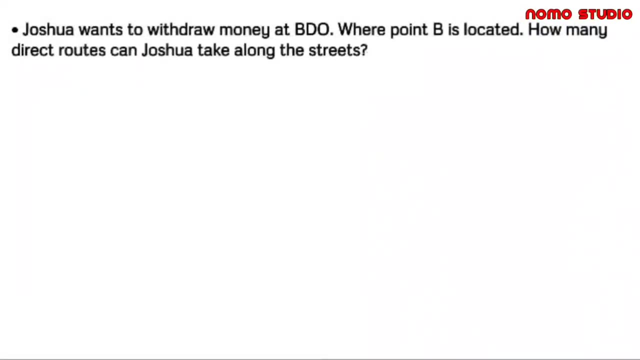 Let's try to solve this one. Joshua wants to withdraw money at BDO, Where point B is located. how many direct routes can Joshua take along the streets? If we try to look at the figure, Joshua wants to travel from point A to point B And the question is: how many direct routes can Joshua take along the streets? 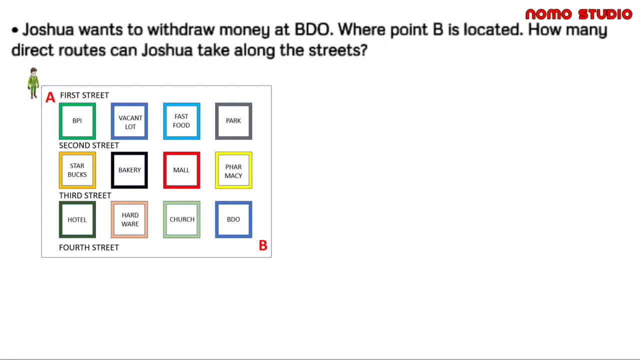 First we need to mark all the intersections on the map. So let's start from point A. If Joshua wishes to withdraw money at BDO through this way- And that is one route- Now if he wanted to go through this way here, This is route 2.. This is also another route, And also this one here. 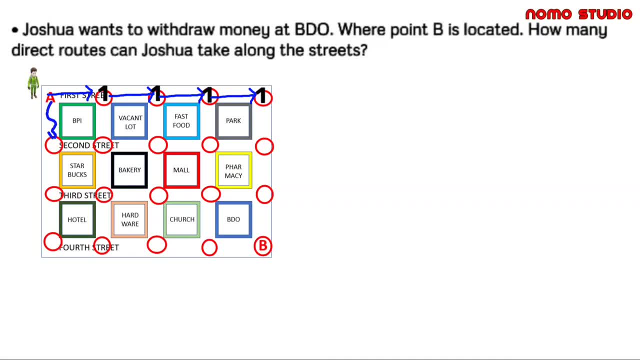 Then if Joshua wanted to go downwards, Then this is also another route, This one And also another route, And this is also another one. Alright, So we already labeled our intersections here For route 1.. And now, What if Joshua wanted to go through this intersection here? 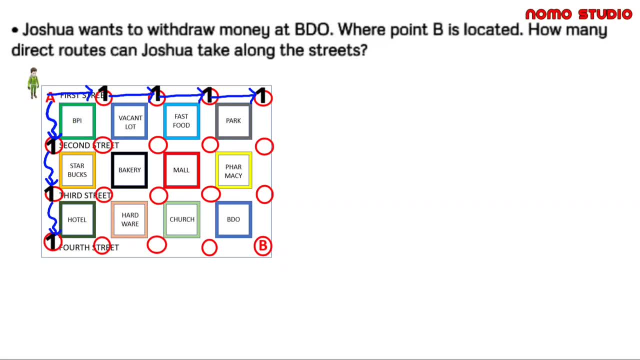 All we have to do Is to add the two adjacent routes, So one route Plus one route. That will give us Two. Now How about here? We have one route And two routes here, So it will give us Three. 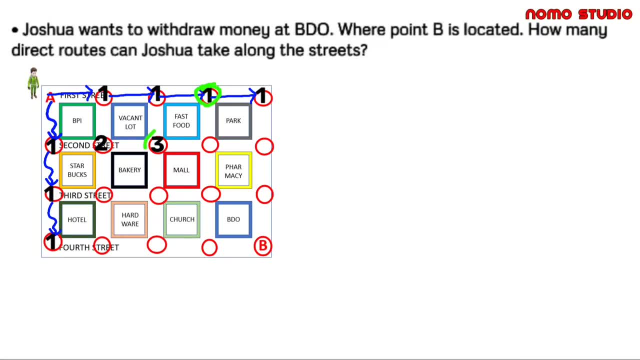 Next, we have One route Plus Three routes, So this is Four. And We have one route here Plus four routes there. It will give us Five routes. Next, we have One route Plus Three routes, So this is Four. 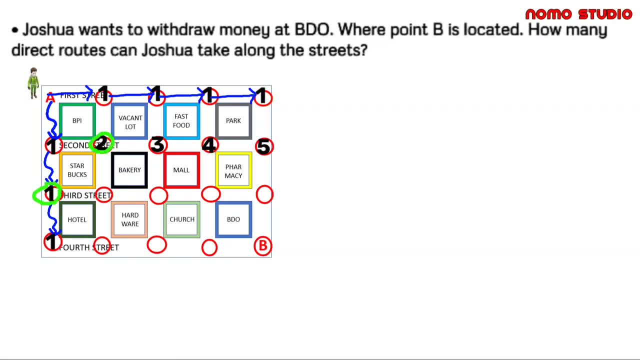 And We have two Plus one route, So it is Three, And also three routes there Plus three routes here, So we have Six. Four Plus Six, That will give us Ten, Then Five plus ten, It is fifteen routes here. 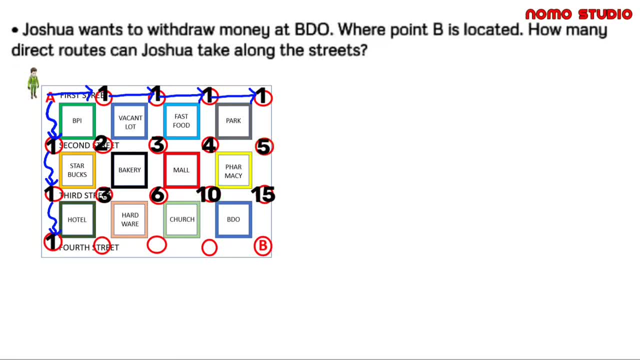 Next we have, By looking at the pattern, This is Four routes, Ten routes, Twenty routes And, lastly, we have 35.. So we already arrived at point B with 35 roots. Therefore, there are 35 roots that Joshua will take him from point A to point B. 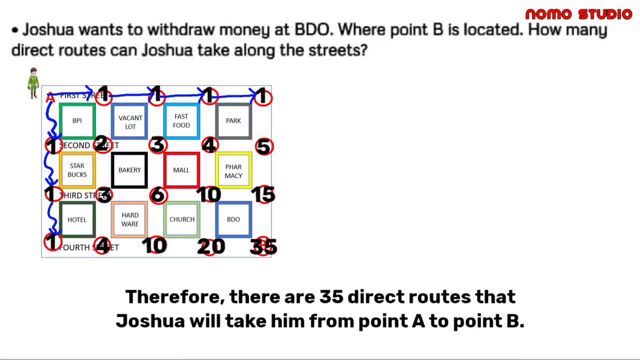 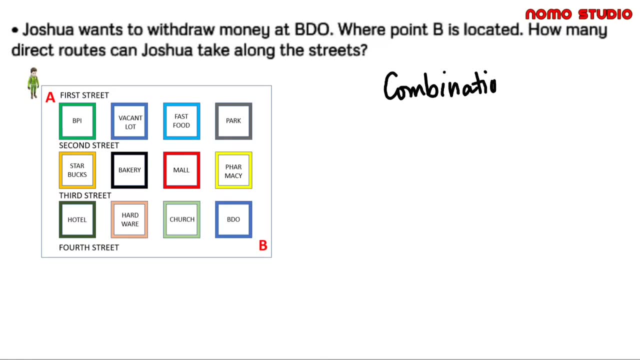 But how about if we will try to solve this one using a mathematical formula, Since we are dealing with counting of the total number of direct roots, so we will use the combination formula for counting and probability. So we have here n taken r equals n factorial over r factorial times the quantity n minus r factorial. 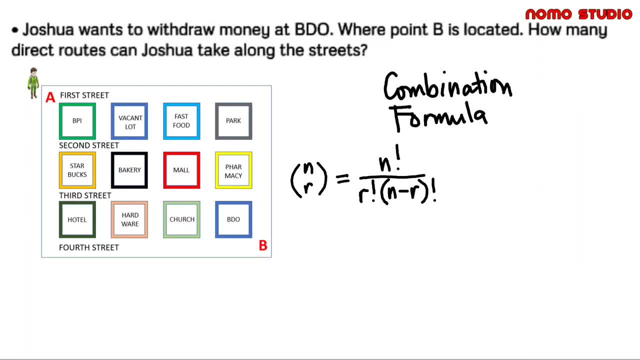 But before that let's put four cardinal directions on the map. This letter n here will be our total number of blocks. going to point B, We have 1,, 2,, 3,, 4,, 5,, 6,, 7, 3 blocks going to south and 4 blocks going to east. 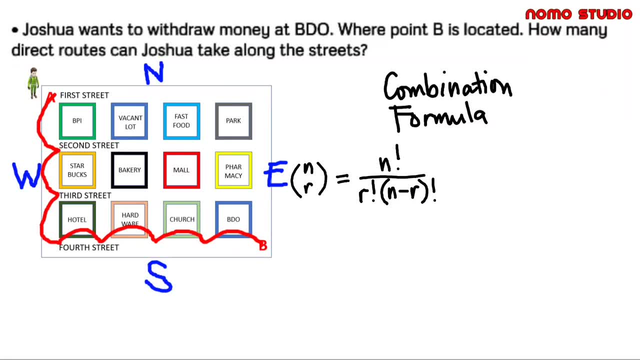 So our n is 7.. To summarize, one direct root is equivalent to 4 blocks going to south and 4 blocks going to east, So our n is 7.. 3 blocks going to east and 3 blocks going to south. 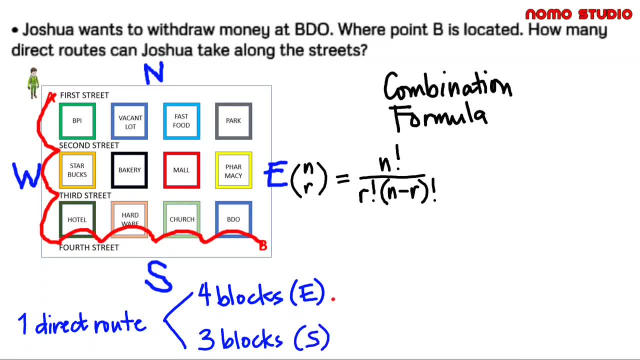 So, to find r, just select one from these two, either 4 blocks or 3 blocks. It will give us the same answer. Note that wherever you go on the map, it will always give 3 blocks of south and 4 blocks of east. considering that you are from point A to point B, 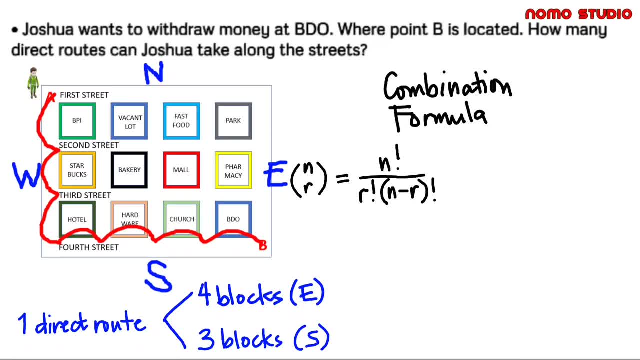 Let's try. r is equal to 3.. 7 factorial over 3 factorial times the quantity 7 minus 3 factorial, So this is 7 times 6 times 5 times 4 factorial Over 3 factorial. then 7 minus 3 is 4 factorial. 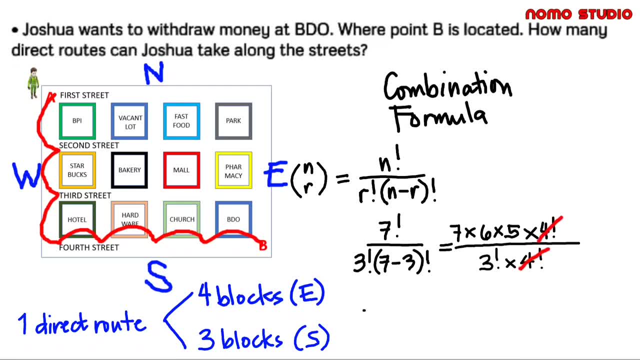 Cancel out 4 factorial. So we have 7 times 6 times 4 factorial. So we have 7 minus 4 factorial 6 times 5 over 3 times 2 times 1.. This is 210 over 6.. So 210 divided by 6 is equal.